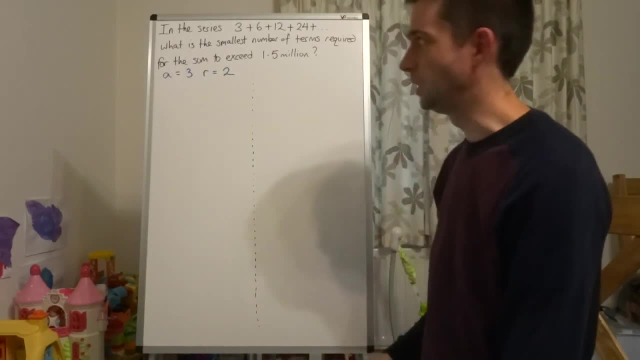 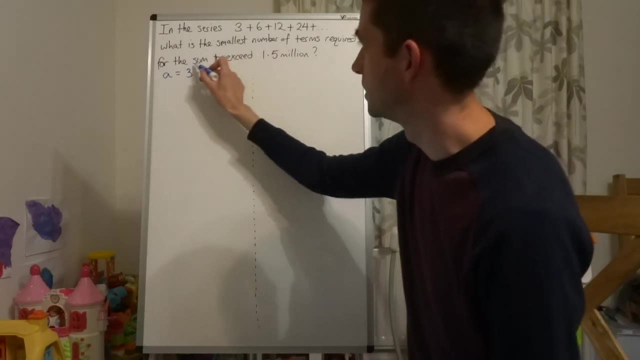 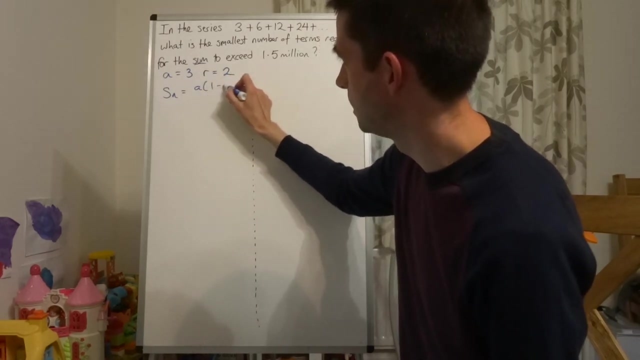 And the first term is a equals 3.. Now we're being asked about a sum, So the smallest number of terms required for the sum to exceed 1.5 billion. So we're going to be using the formula: sum to n equals a times by 1 minus r to the n. 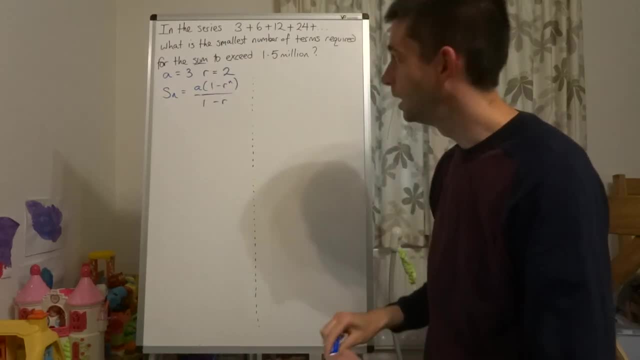 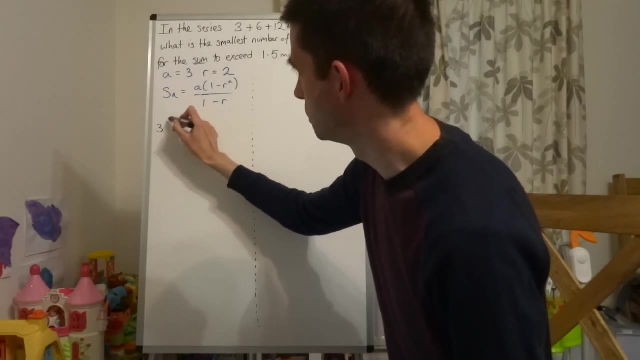 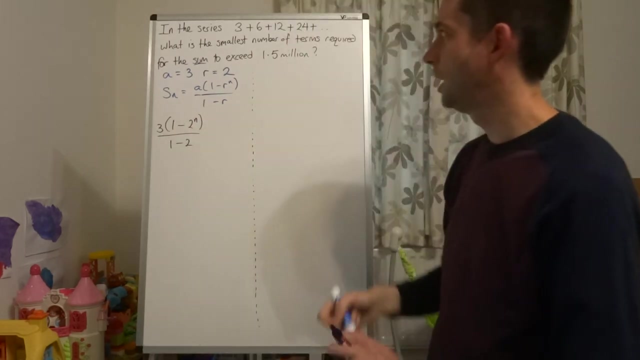 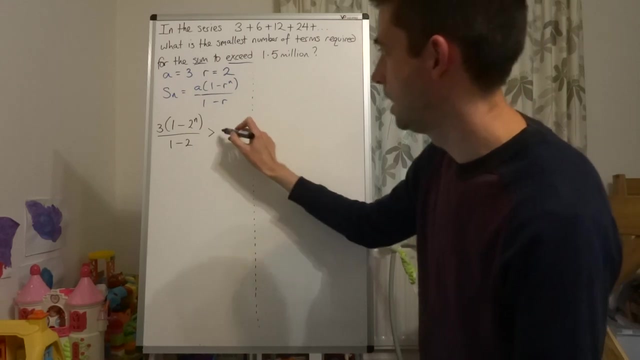 So let's begin by using that formula with the values that we know. So a is 3.. 1 minus 2 to the power of n over. 1 minus 2 exceed greater than more than So the inequality symbol is going in this direction: initially 1.5 million, So 1, 5 and then 5 zeros. 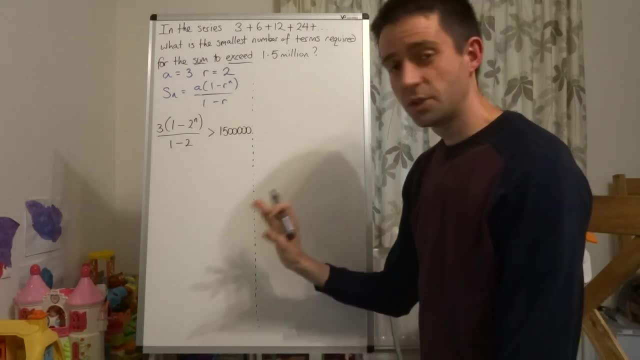 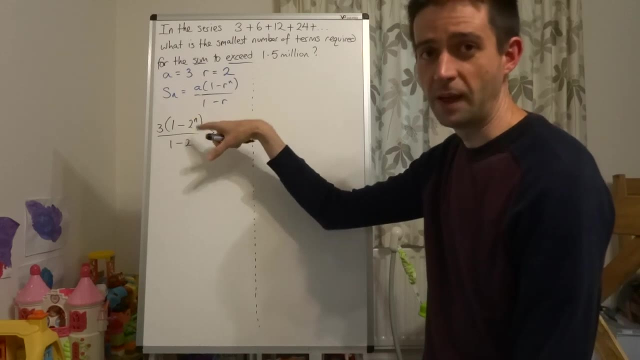 Now what you must not do is multiply this bracket out, Because what people tend to do is they'll say: oh, it's 3 minus 6 to the power of n, And it's not. You cannot times that 2 by that 3.. 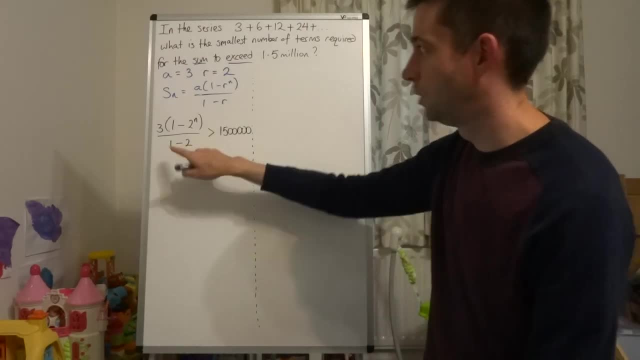 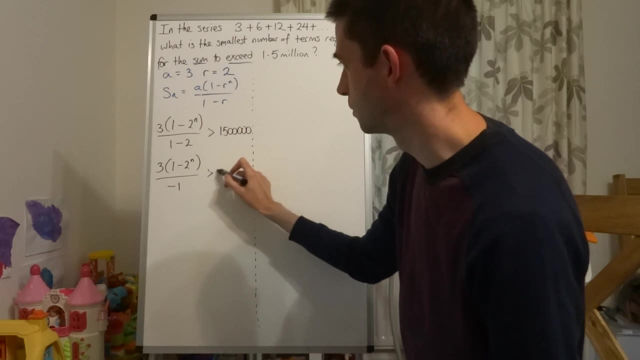 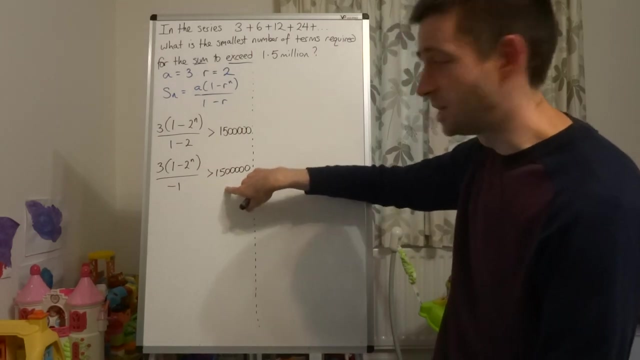 So what we do instead is we say that 3 lots of 1 minus 2 to the power of n over negative 1 is greater than 1.5 million. We're then going to multiply both sides of this by negative 1.. 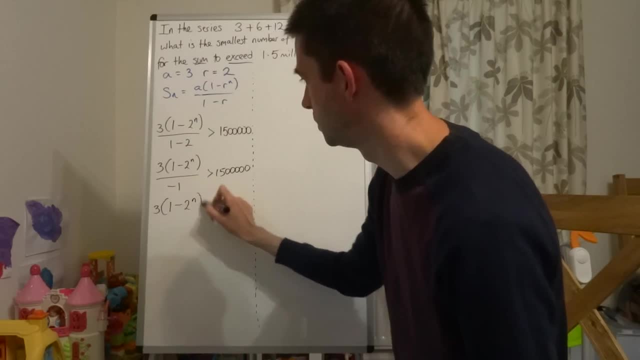 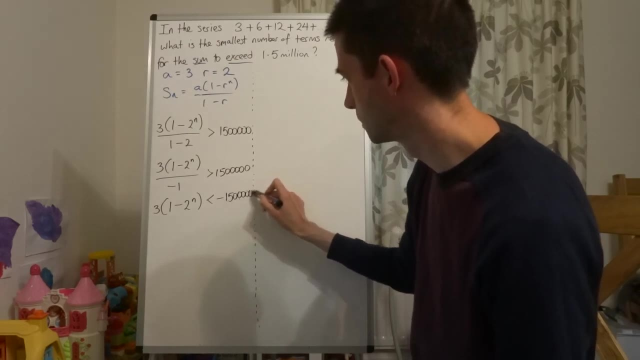 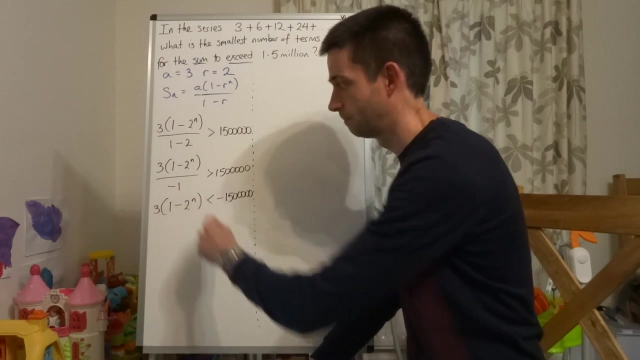 So we're going to have 3 lots of 1 minus 2 to the power of n is less than negative 1.5 million. And that inequality has changed direction because I've multiplied both sides by a negative. So again I said we're not going to expand those brackets out. What we're going to do is we're going to divide by 3.. 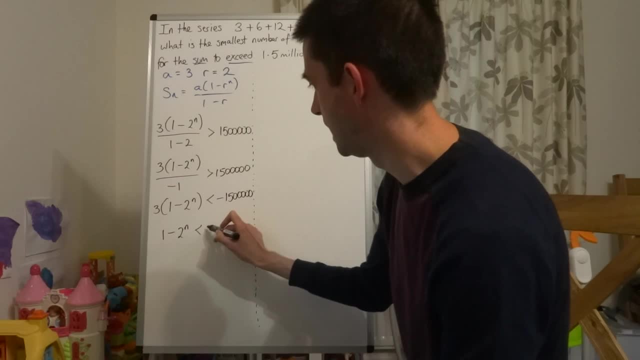 So we're going to have 1 minus 2 to the power of n. So we're going to have 1 minus 2 to the power of n is less than negative 500,000.. Dividing this by 3 as well. 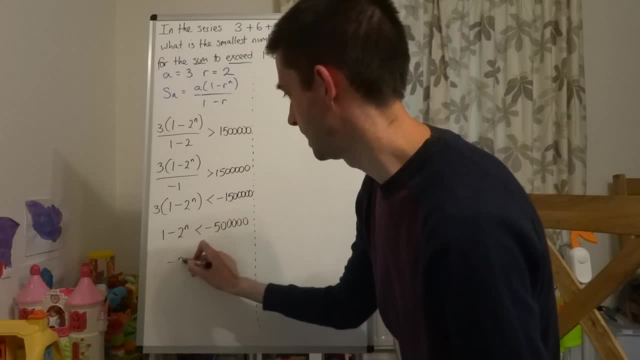 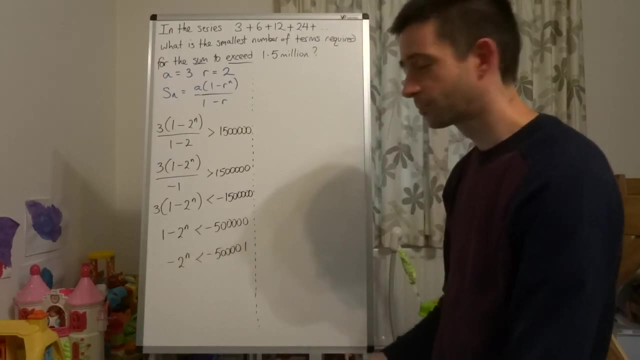 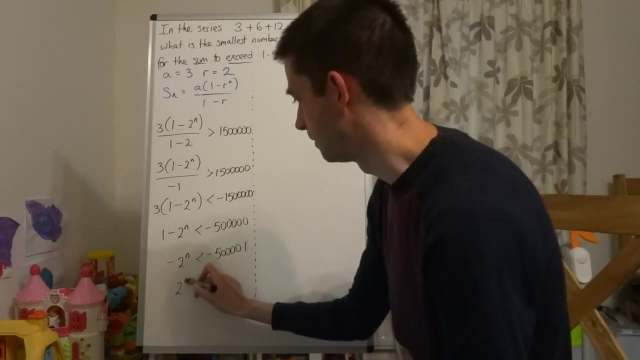 We're going to subtract that 1.. So we're going to have negative 2 to the power of n is less than negative 500,001.. And then, because we've got two negatives, we can divide both sides by negative 1 to get 2 to the power of n. 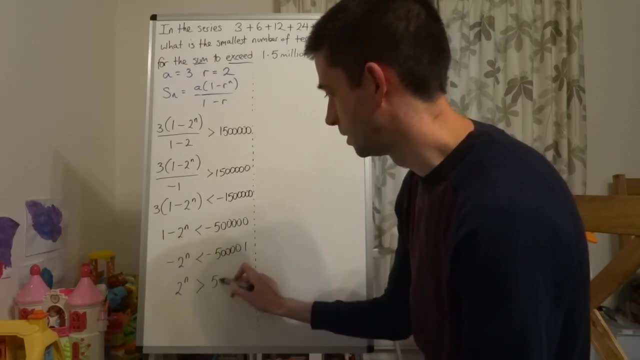 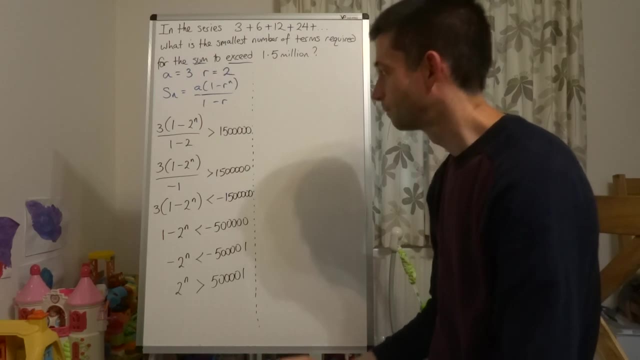 Now, crucially, that will change the direction. So we're going to have 2 of the inequality, So 2 to the power of n is now greater than 500,001.. So I just jot that again up here so that we can work from that. 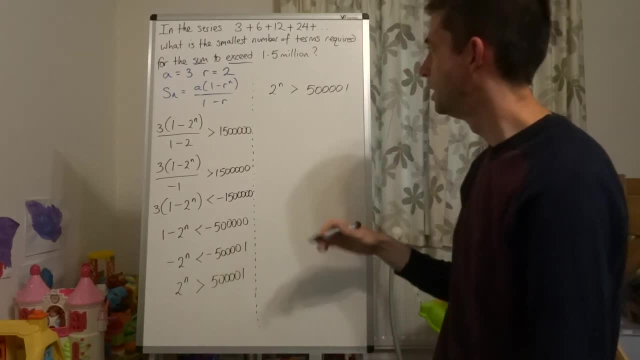 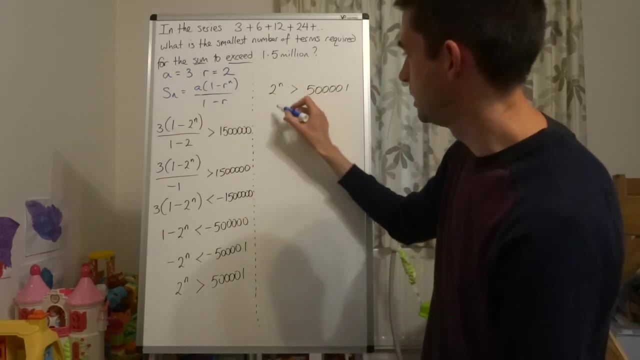 2 to the power of n is greater than 500,001. and now it's a case of how do we solve for n? Now you might be tempted to say: oh yeah, I see this, Mr Sudden. It's base power, So it's log base 2 of 500,001.. 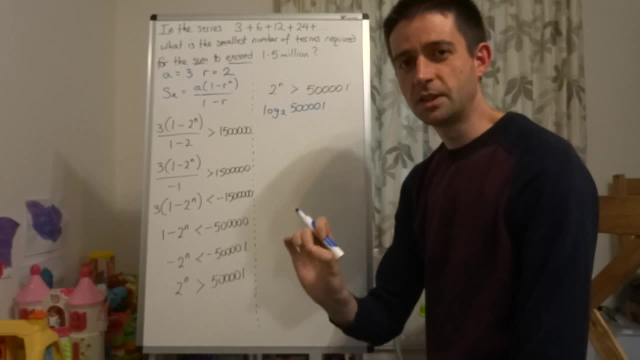 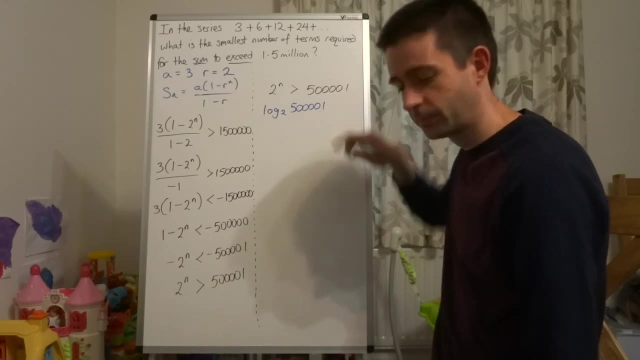 And that's going to give me my odds answer, And that's great, except that we need to keep the inequality symbol in there and we need to know well, is it more than this number or is it less than this number? So, 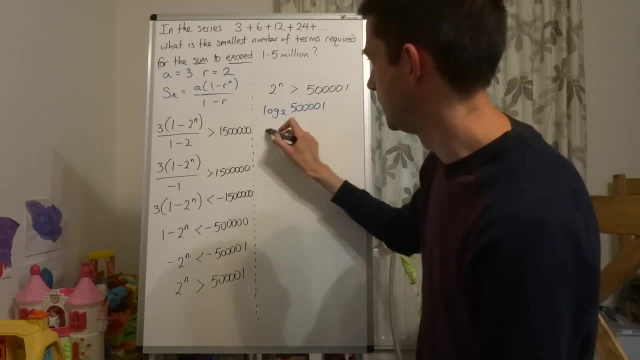 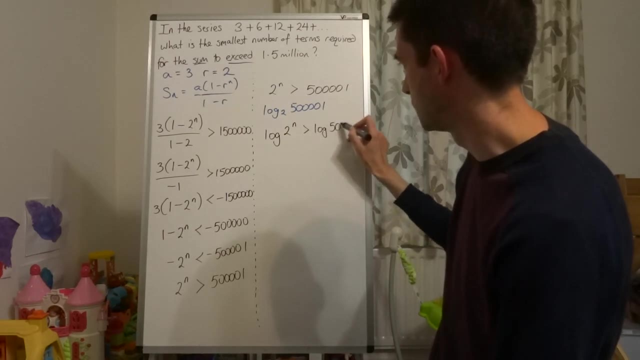 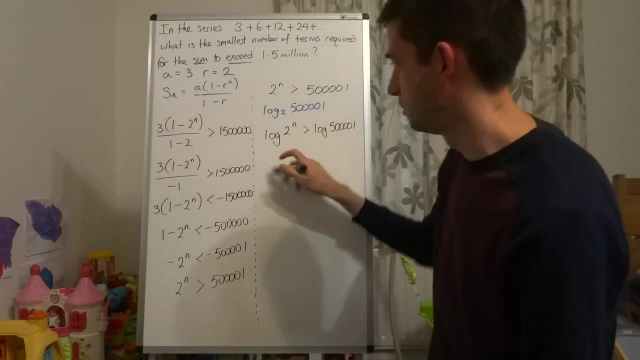 my preference, rather than jumping to this, is to take logs of both sides and say log two to the power of n is greater than log of 500,001.. We can then use the powers rule of logarithms and place the n in front of log two, still greater than log 500,001.. Now 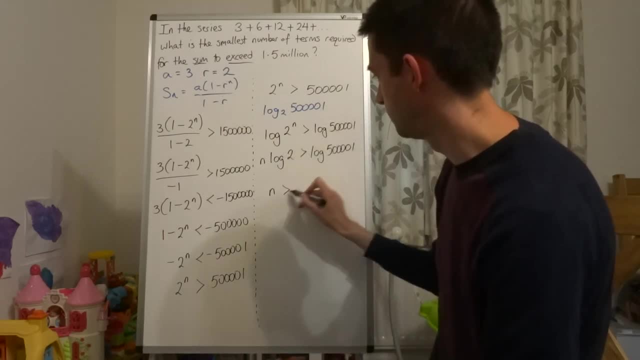 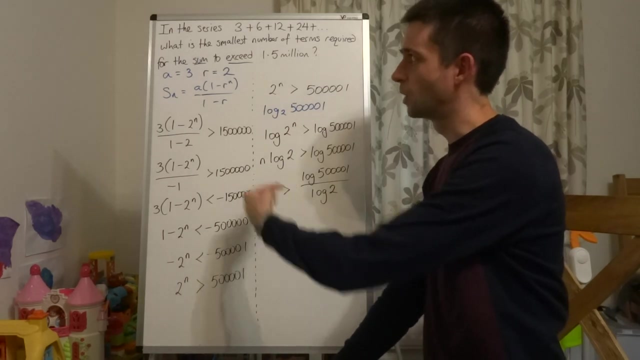 log two is a number, which means that we can divide both sides by log two to get log 500,001 over log two. Now let's just pause for a minute to check that this is sensible. We've been asked for the number of terms required to exceed log two, So we're going to take log. 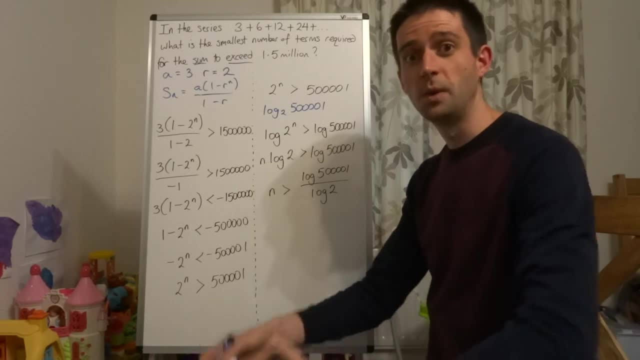 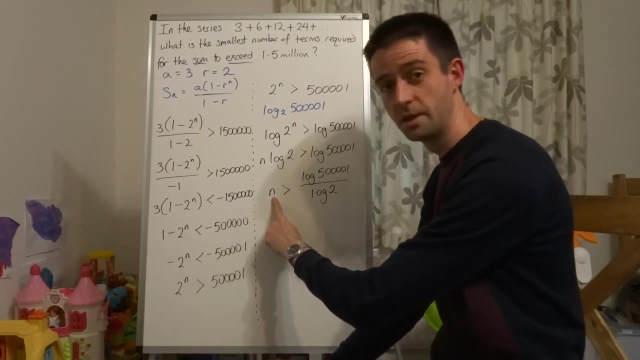 two, which is greater than log 500,001.. This is a number that we can check here. That's a certain value. Now, you would expect that to be after we've had a certain number of terms. So, more than this number of terms, And this inequality is saying that n the 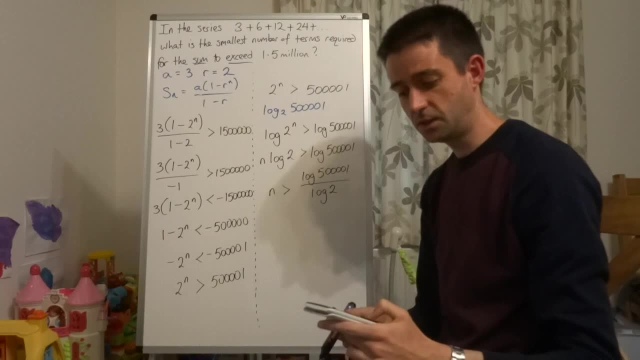 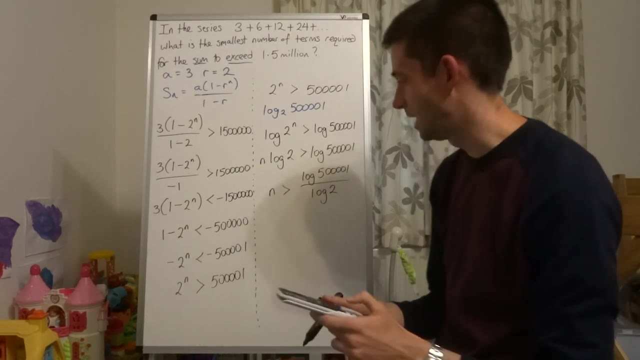 number of terms is more than this number. We're happy with that. That makes sense at this stage. So all I need to do now is using my calculator and the log button defaults to base 10, but it doesn't actually matter what base you use. 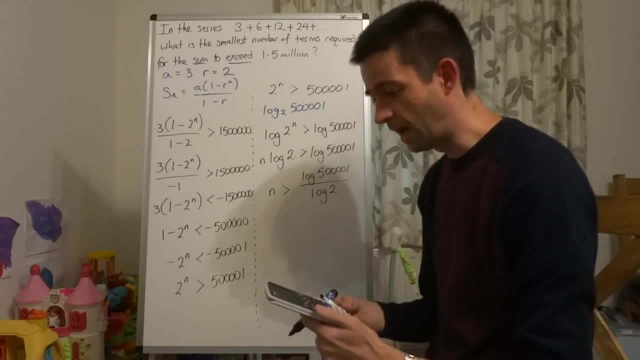 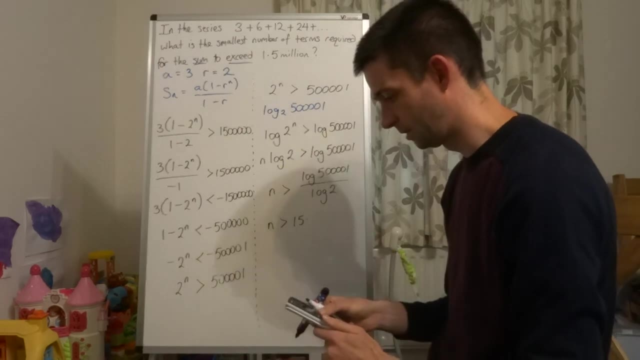 Let's just try and do this again: Logarithms learn, it will work with learn as well. And what we get is n is greater than 15. point. Hang on, I've not put enough zeros in there. There we go. 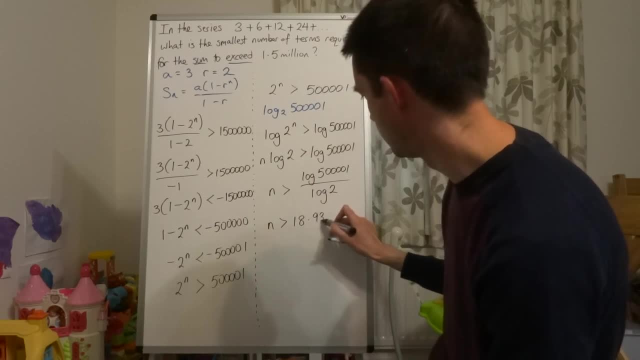 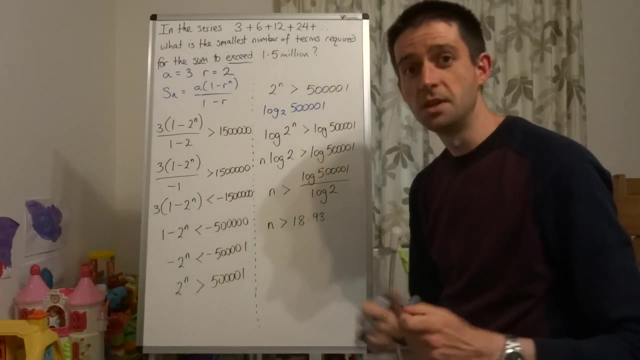 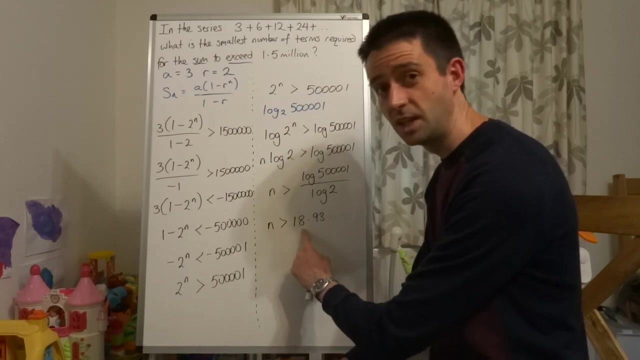 n is greater than 18.93, etc. etc. So let's just think about what n represents. n represents the number of terms in a sequence, So that can only be an integer, a whole number. So if n is greater than 18.93, then n must equal 19.. 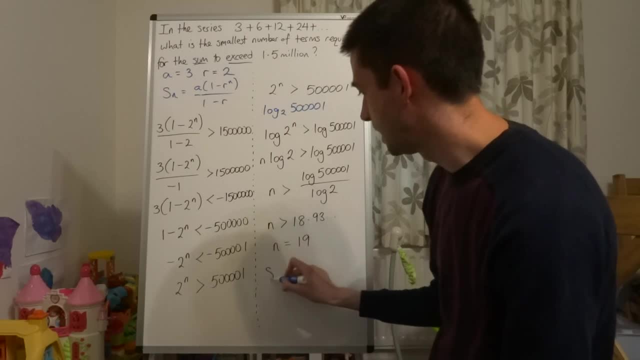 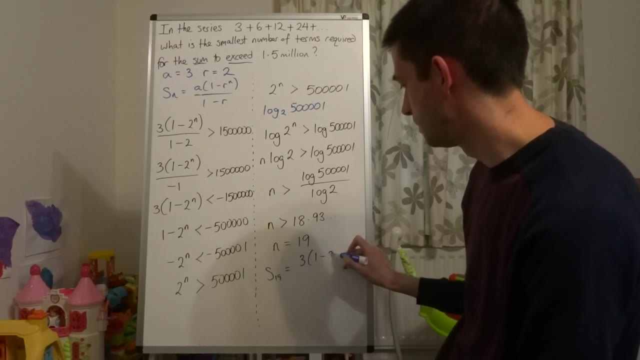 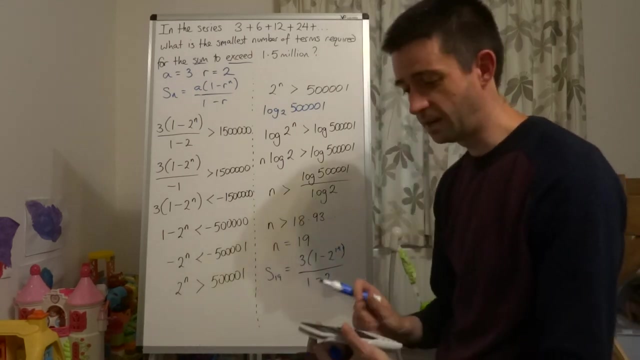 And if you just wanted to check it's worth doing. You could say: sum to 19 is a, which is 3,, multiplied by 1 minus 2, to the power of 19.. All over, 1 minus 2.. Just check, that's greater than 1.5 million. 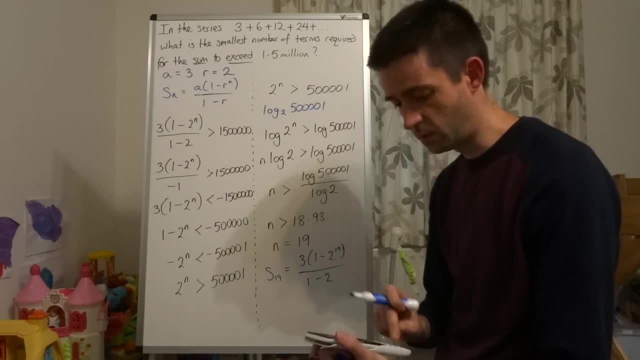 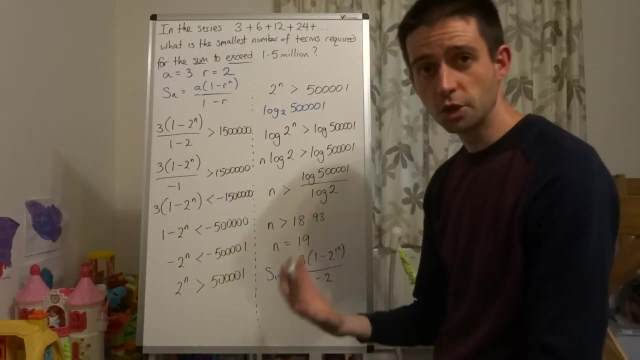 I'm just going to do it now. So 3 multiplied by 1 minus 2 to the power of 19.. All over, negative 1 comes out as just over 1.5 million. So there we go, Just while I'm here. something to be aware of is if this had been a decreasing series. 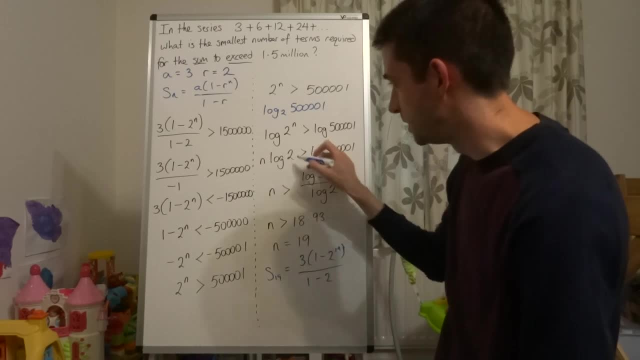 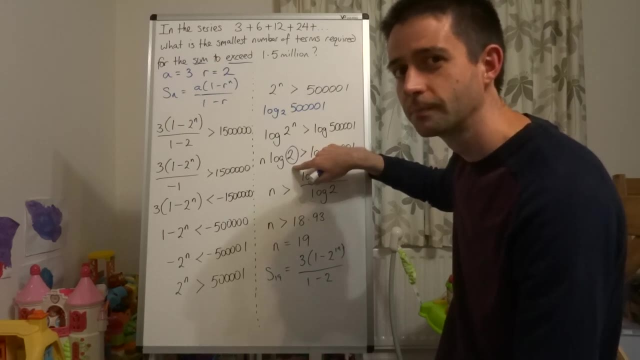 so your common ratio had been 1.5.. If this had been a fraction, then what would have happened is at this stage here. if you have a fraction, think about what is log of a number less than 1.. Say, for example, if, instead of 2, this had been 1 third, you'd have log 1 third there. 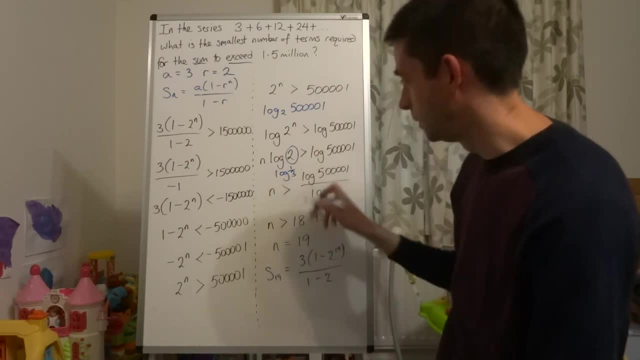 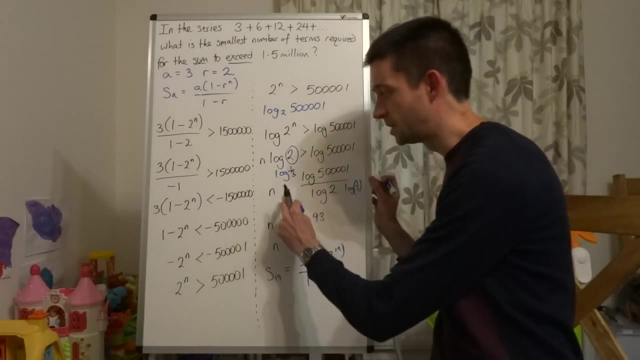 Well, log of 1 third is negative. So if you've been dividing in this next step by log of 1 third as well as dividing by log of 1 third, the inequality would have to change direction Because you're dividing by a negative. 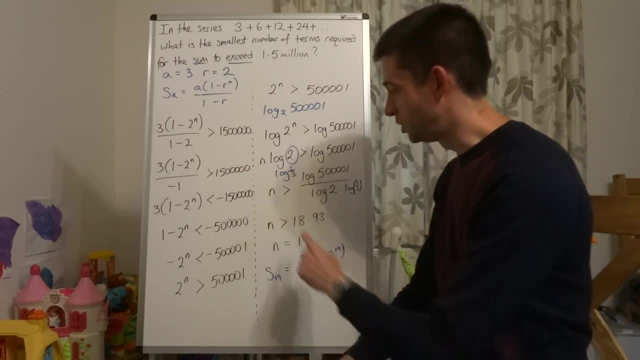 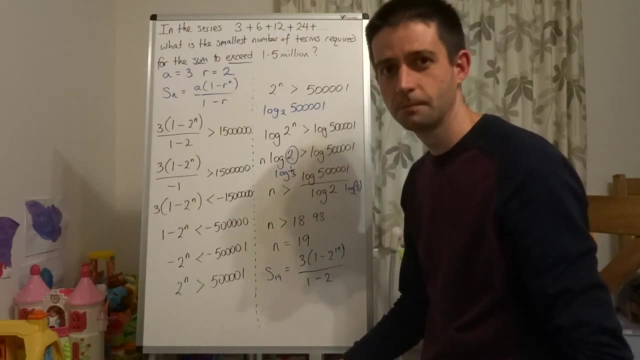 And it's little tricks like that that make it important to just consider at this stage, am I comfortable that the inequality is going in the right direction for the context of the question? There you go, Job done. Thanks for your company.